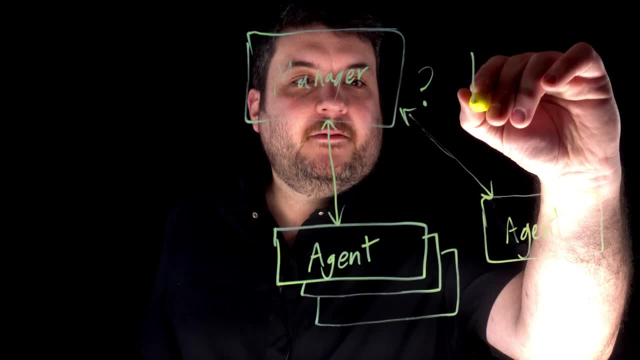 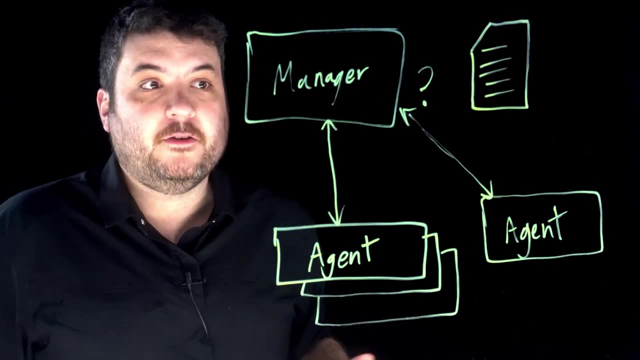 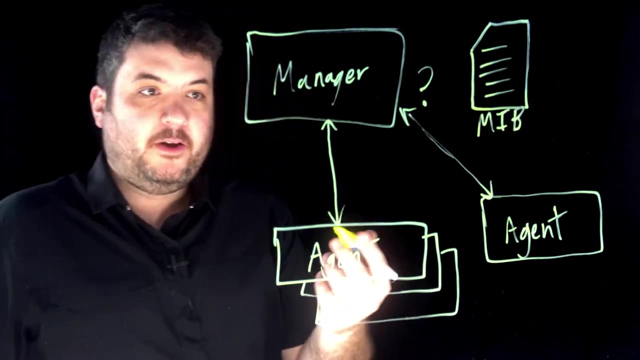 How do I talk to this thing? Well, that's what the MIB file is. The MIB is actually a plain text file. It's an ASN.1 notation And it contains all the instructions That that manager is going to need to resolve all those questions about what this device can do and how to talk to it. 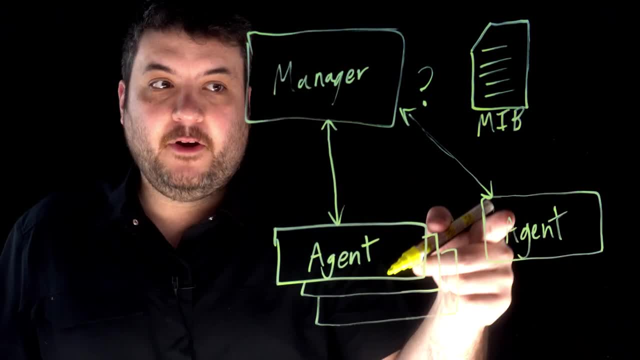 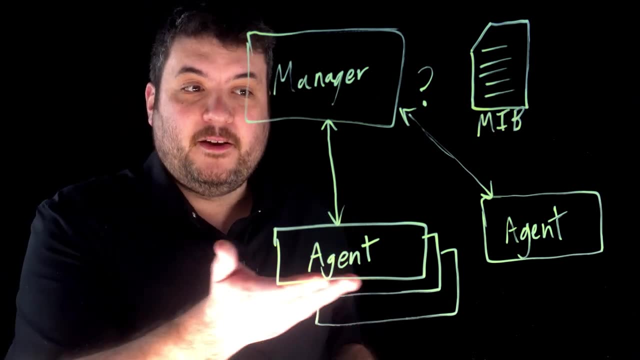 So the MIB should be provided by the manufacturer of your agent. It's just like a driver file: If you bought something, that device's manufacturer should give you a driver file. Well, the supplier of your SNMP agent ought to give you a MIB. 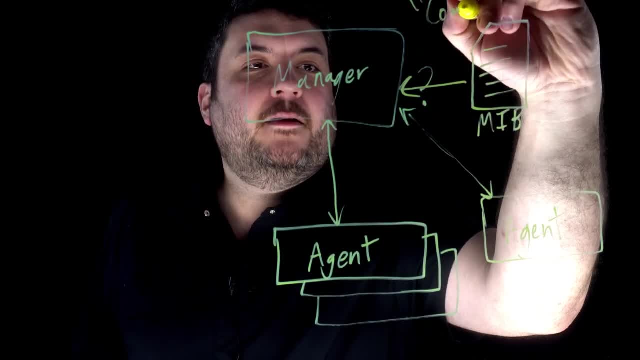 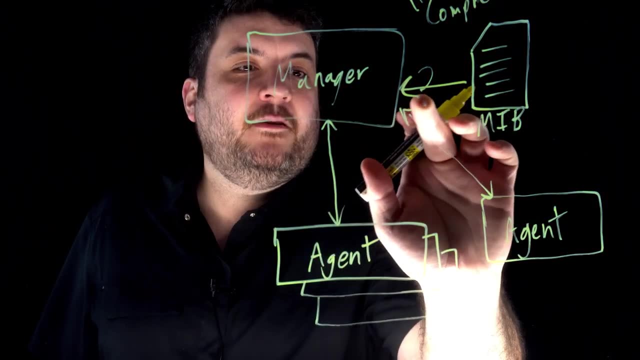 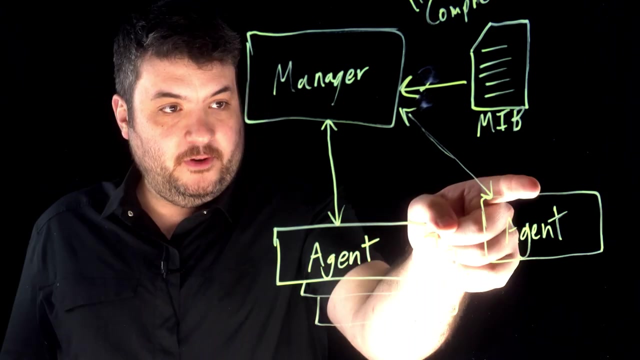 So you do what's called compile that MIB into your manager And at that point there's no longer any issues. If there's any question, it can understand what's going on with that agent. I will warn you, though some manufacturers of agents may say: oh yes, we support SNMP absolutely. 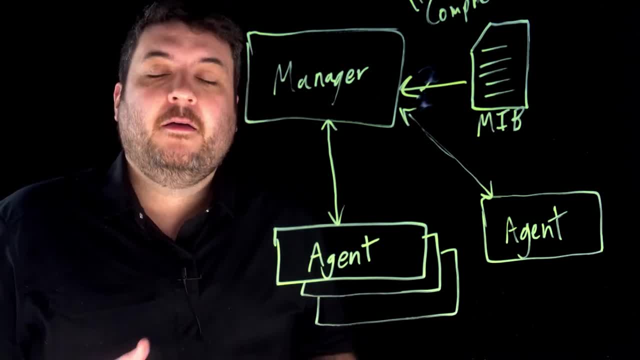 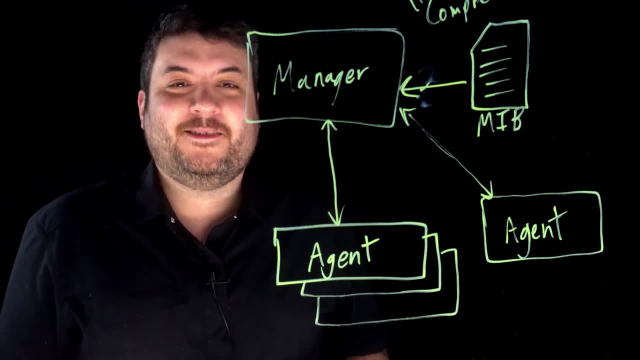 But they may be protecting, from a business standpoint, their own system that is non-SNMP, that uses a proprietary protocol, And to do that one effective way is to not freely distribute a MIB. So be careful that you don't get into that trap if you're considering a purchase. 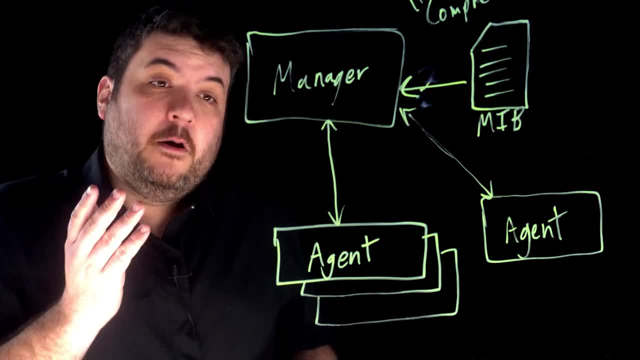 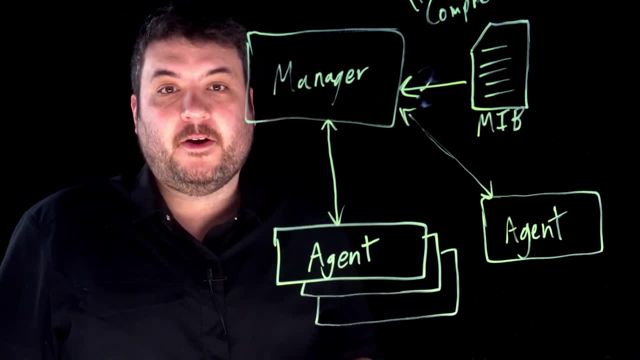 Talk to your manufacturer. Make sure that the MIB is readily available. One other thing of note: Some masters and managers are getting smarter, And so just an example pulled from the DPS environment: Our team on master station is equipped with what we call device modules. 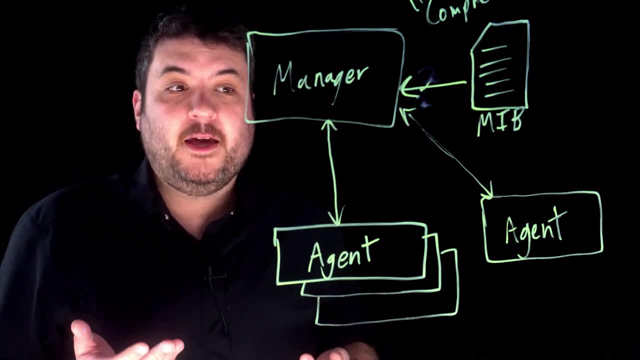 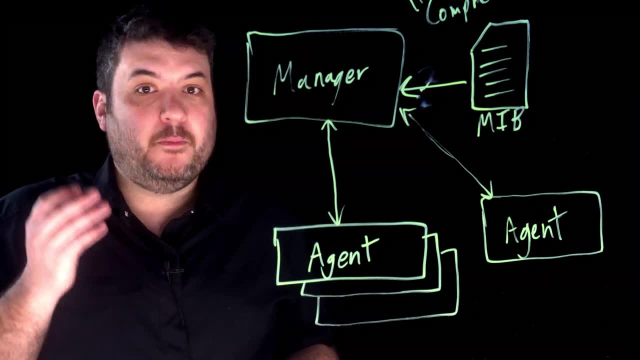 If you have a device module, your manager may already understand intrinsically how to work with certain common agent types, And if you have that, you may not really need to use a MIB at all. The manager might be pre-equipped. So as that model continues to take hold in the industry, you may see less and less need for MIBs. 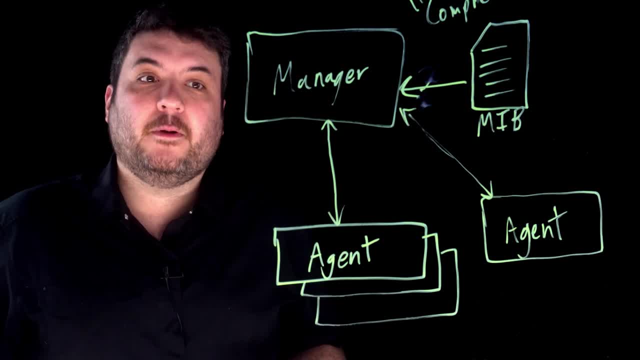 But if you're loading a non-standard agent, you're going to need a MIB. So you really need to make sure you have that MIB file available so that your manager can get it compiled in there and understand how to talk to that agent. 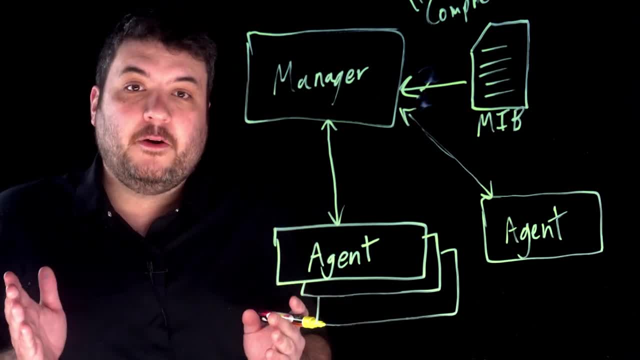 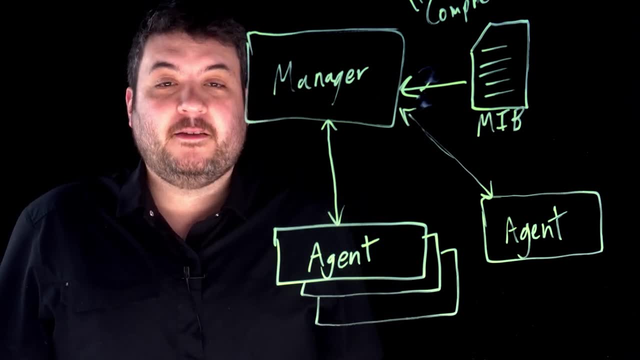 I hope this cleared up a few things for you. Please, if you found this video helpful, click the like button and subscribe to the channel so you can get more videos like this one, And until next time, I'm wishing you excellent network reliability. Thank you.